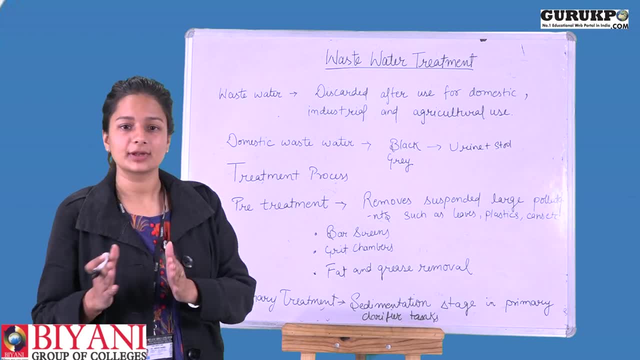 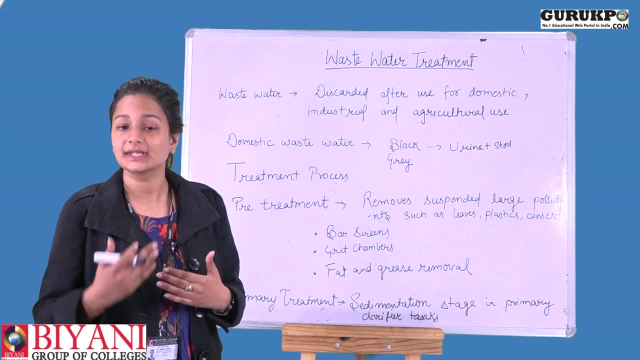 A processing of any thing is done. That is why the processing of waste water, out of which most of the heavy waste is done. That is why most of the heavy waste is done. Most of the heavy waste is done, We remove it. 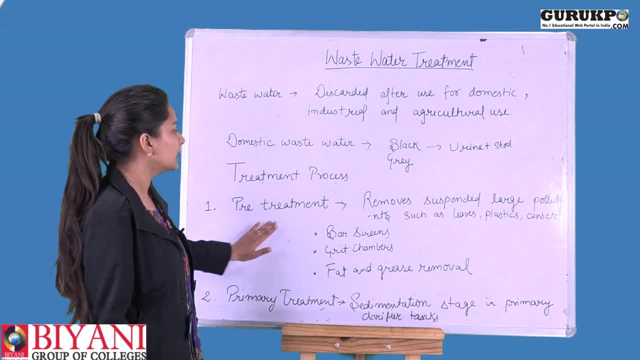 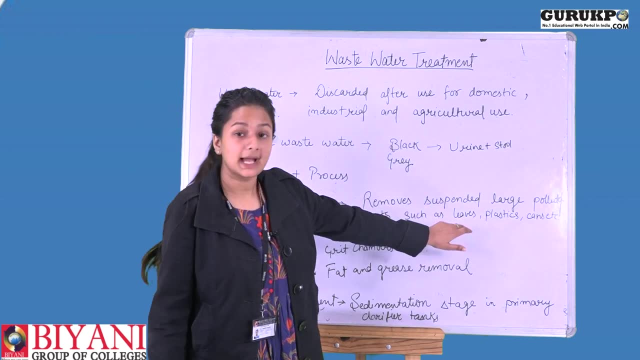 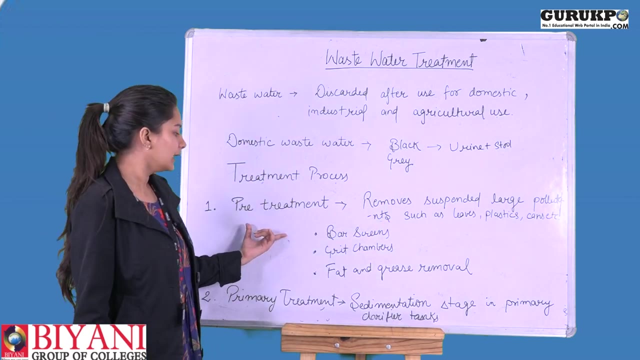 That process is called pre-treatment process. In pre-treatment we remove all the suspended particles, suspended large pollutants, such as leaves, plastic or aluminium cans etc. So we do pre-treatment with the help of three processes or three kinds of things. 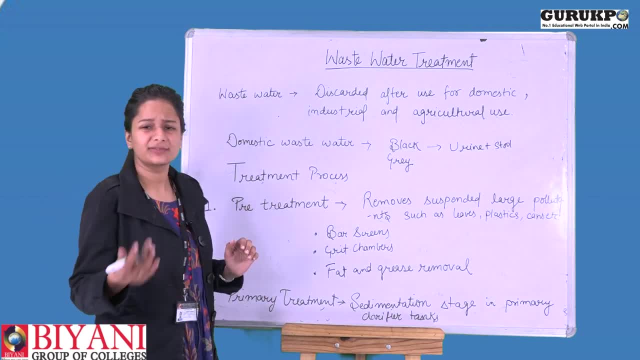 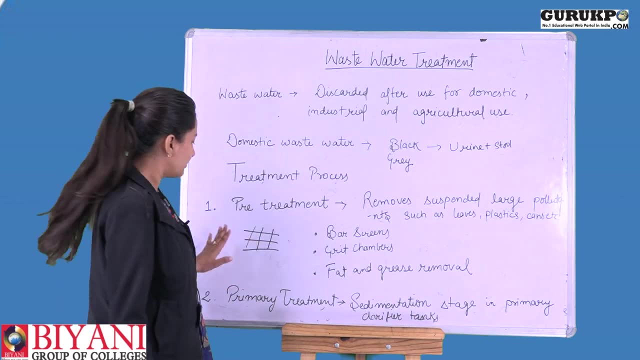 First of all, bar screens. Bar screens are made up of steel or iron. Bar screens are made up of steel or iron. Large bar screens like these. They act as filters. Bar screens act as filters. Through bar screens, we pass our polluted water. 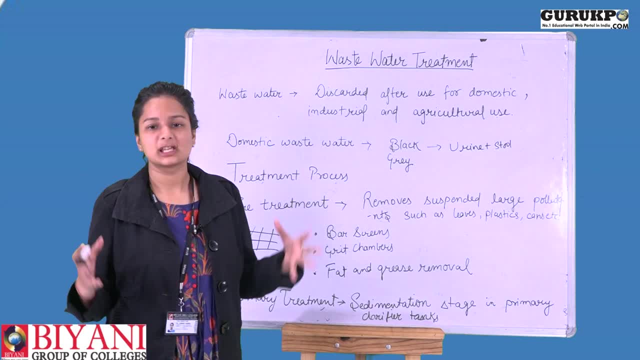 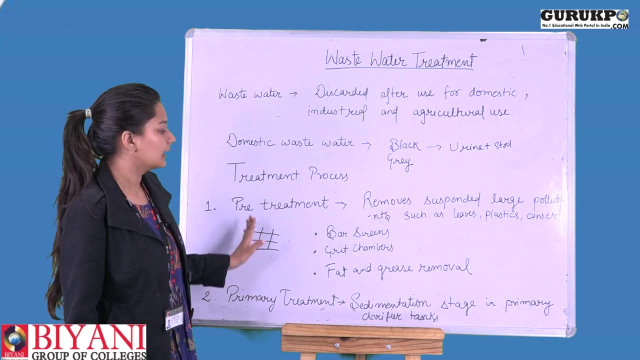 As we pass the polluted water, most of the suspended particles get accumulated on one side of the bar chambers. It is as we pass the polluted water, most of the suspended particles get accumulated on one side of the bar chambers and our clean water get passed through it for the further treatment processes. 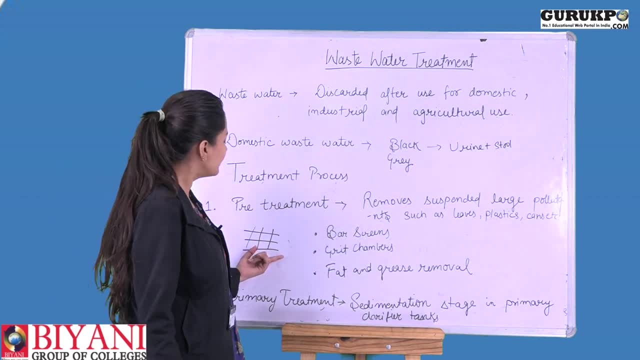 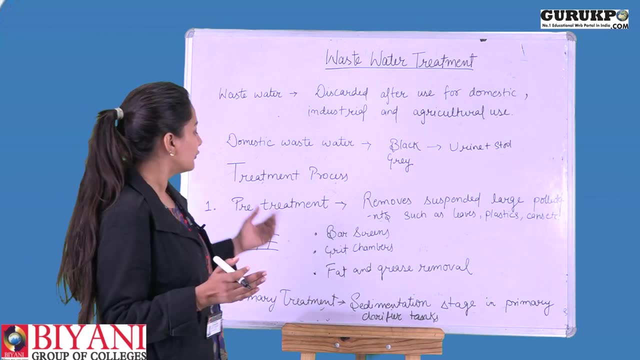 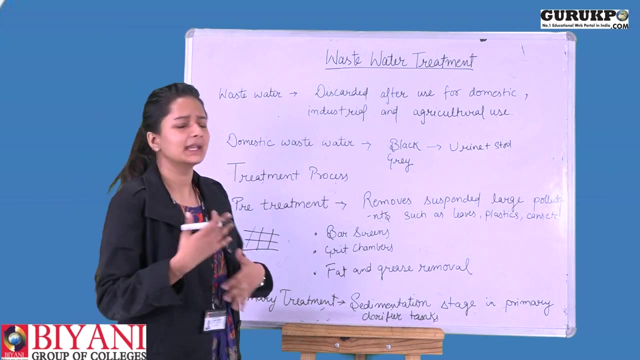 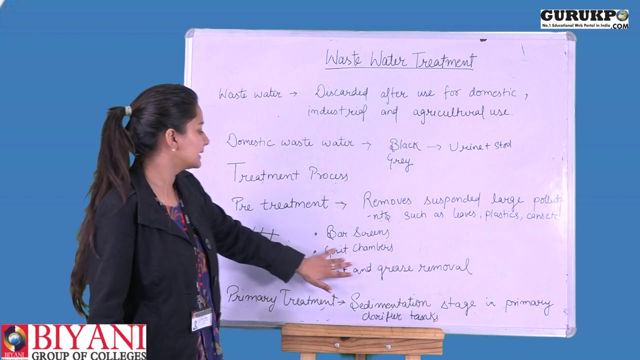 Next are greet chambers, bar screens. we pass our wastewater in great chambers. green chambers are like ponds or tanks okay, in which we add greet. greet is sand or gravels okay, which makes our suspended particles or any other pollutants to get stick to them or get sedimented. so this great chambers are basically have a principle. 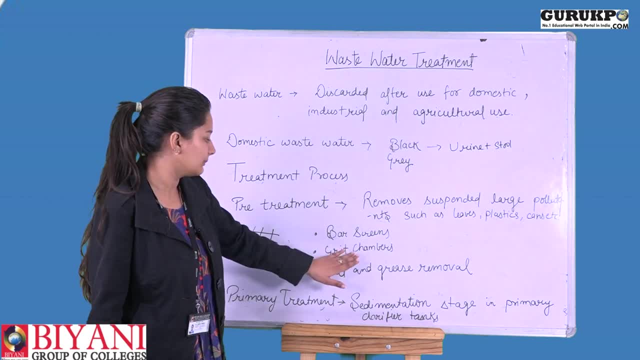 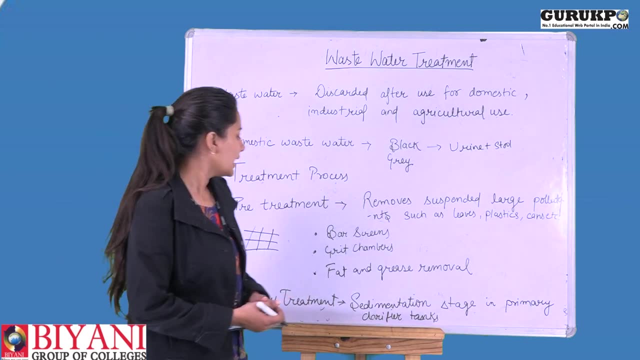 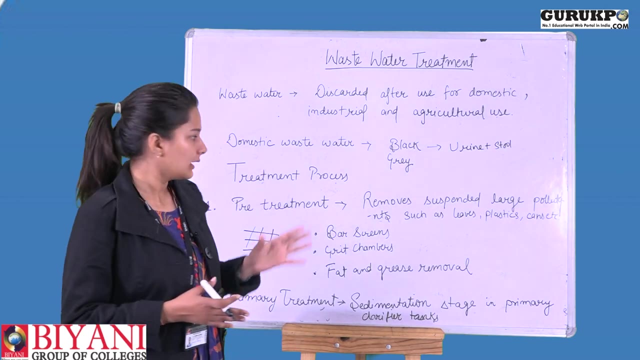 of sedimentation. it means all the pollutants will get sedimented in great chambers with the help of greet. next is fat and grease removal. okay, after we have removed our suspended particles, so in as we can say that in our domestic water, waste water, grease or fats are also available. so it's important to 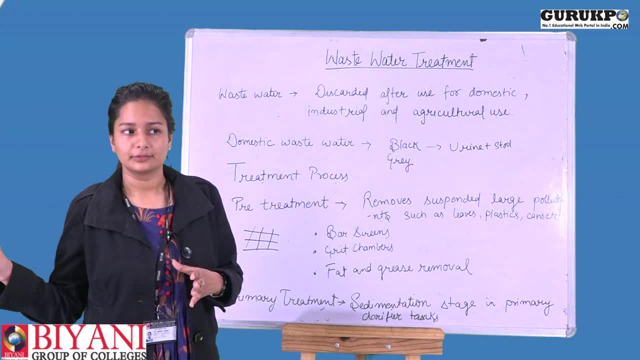 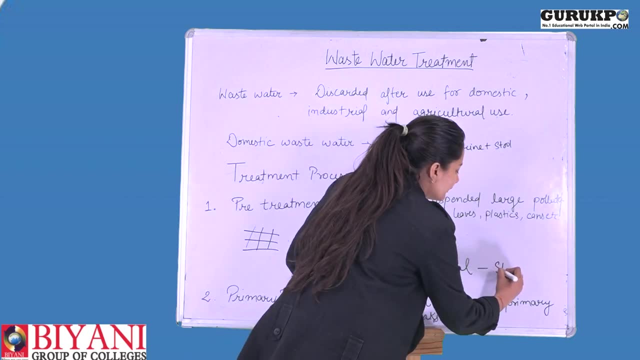 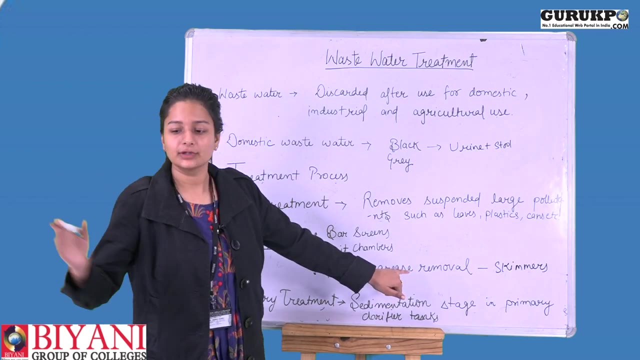 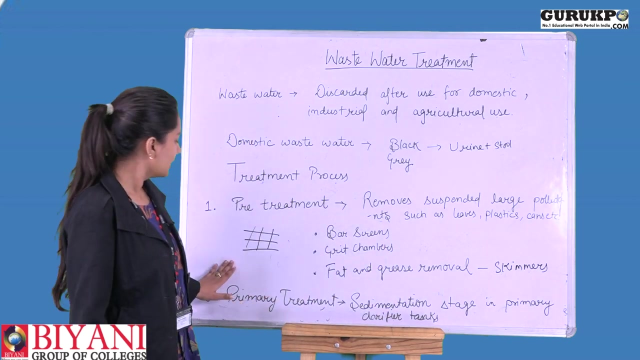 remove them before discharging in any water resource. so we remove fat and grease removal with the help of schemers- okay, with the help of you schemers. schemers make fat and grease to float on the surface of water and with the help of air flow we make that fat or grease separated from the tank. so first, 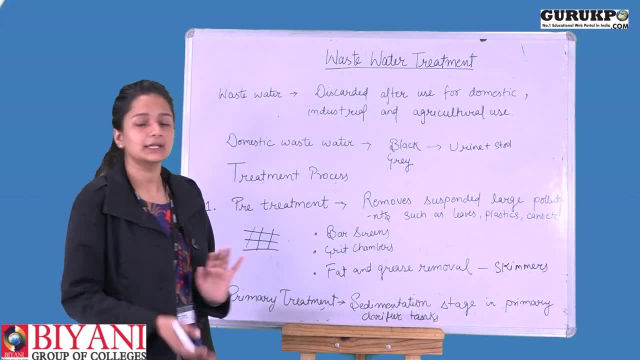 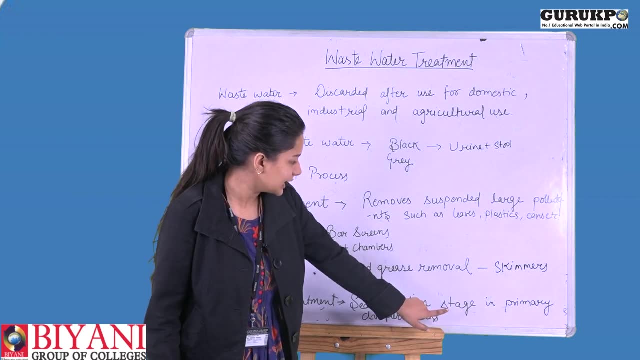 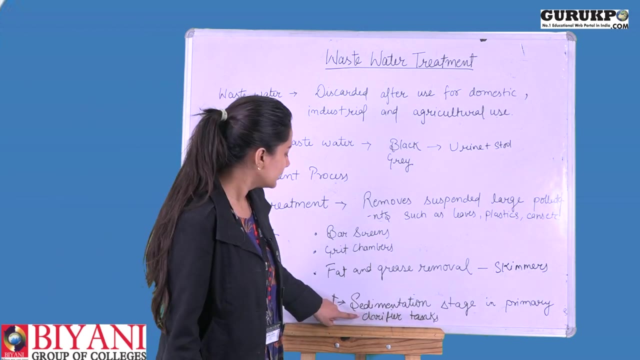 has been completed. next is our primary treatment. primary treatment is also completely based on sedimentation, so this is our kind of sedimentation stage in primary clarified tanks. the tanks which are being used for treatment are in this process are primary clarifier tanks, means after passing through the 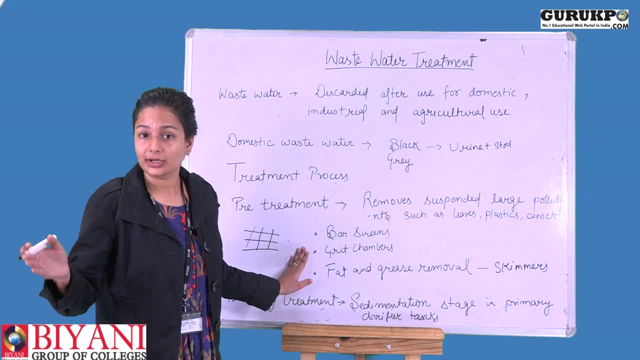 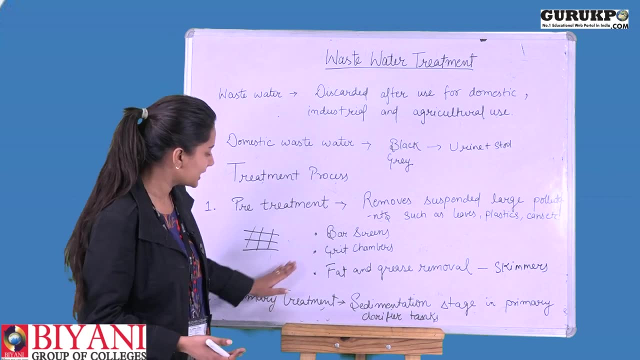 great chambers. great chambers will make the speed of water very slow. agar speed slow ho jayegi toh hamara sedimentation ka process ki rate bhat jayegi isliye jaise water, waste water, hamara primary clarifier tanks mein. 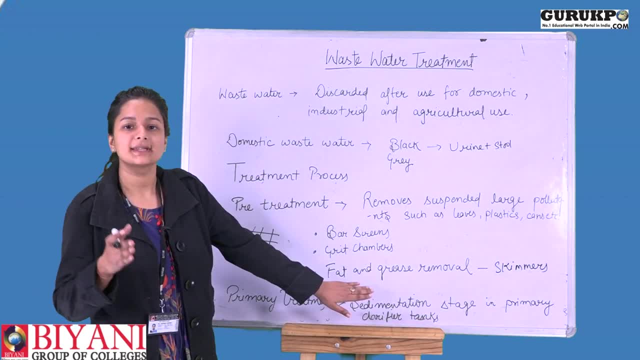 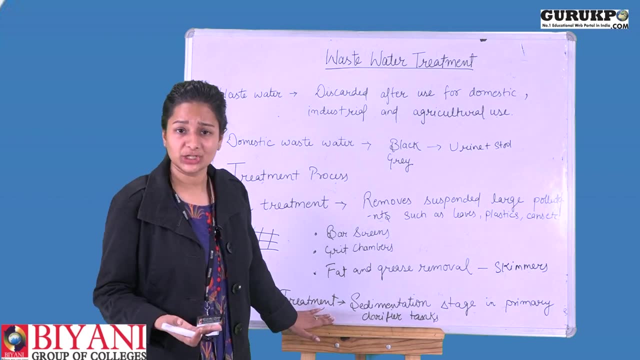 aayega wahan pe flow rate, jo hai wo kum ho jayega or sedimentation increase ho jayega. further is may primary heat treatment, may hum flocculation or coagulation ke liye chemicals we add karte hain, jo suspended ya suspended. 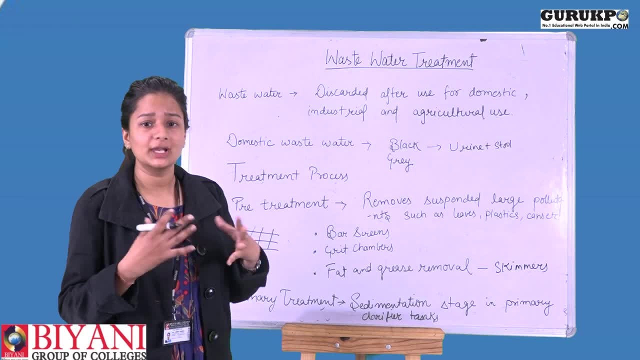 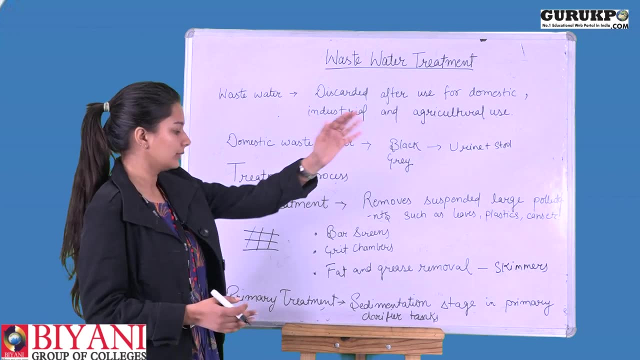 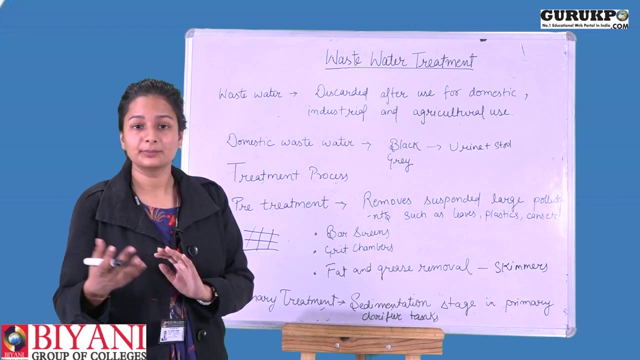 small particles kaih sakte hai ya fir dissolved particles jo coagulation ki through ya coagulating agents. jab ham add karenge, toh unhe precipitate karke, unhe water ki upar float kira dega, as the precipitants or coagulant coagulated. 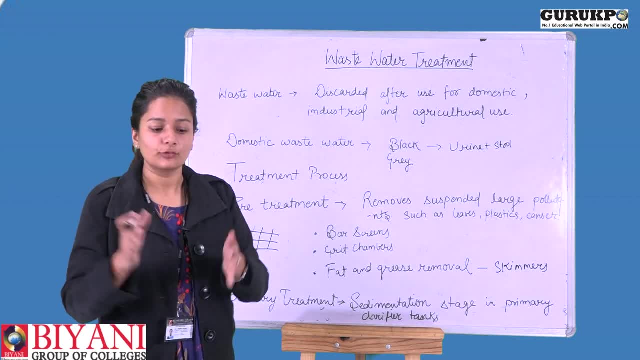 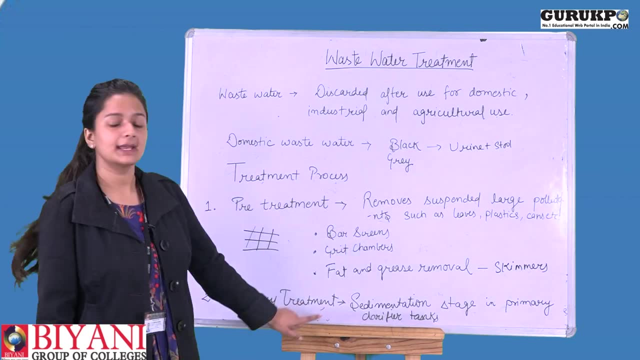 material will float on that as we pass through the coagulation and coagulation pass air from the tank wo air ke saath mein saare hamare. suspended particles separate out ho jayenge. so the primary treatment is totally based on our coagulation, flocculation and sedimentation. so, as we have seen, our 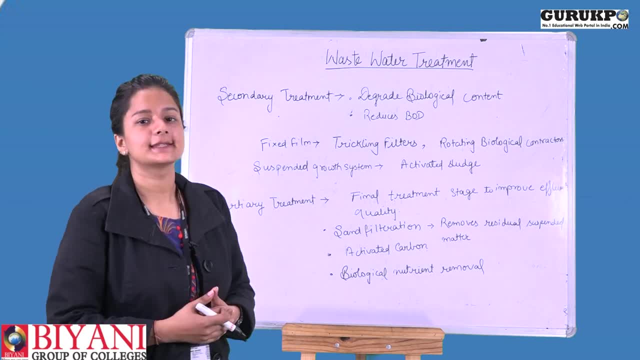 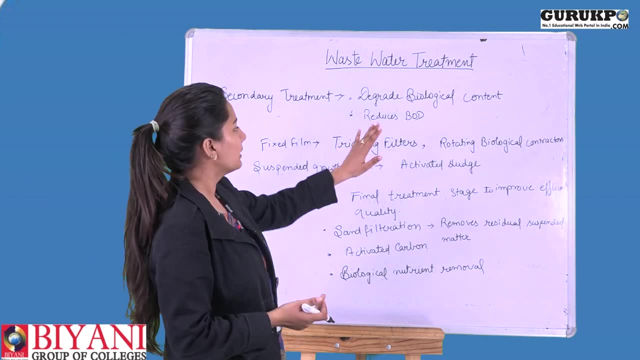 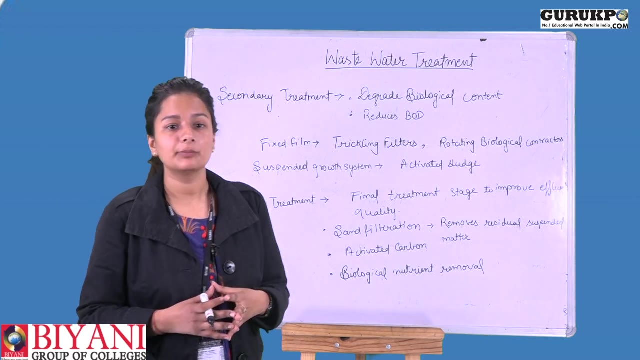 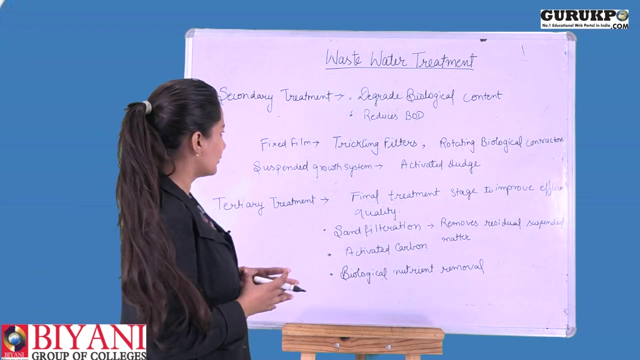 primary treatment. after try a primary treatment, the next step comes our secondary treatment. so secondary treatment is totally is biological treatment, or its synonym is biological treatment. in this, with the help of microbes, we degrade our organic matter which is present as pollutant in our wastewater, so we degrade biological content in this. 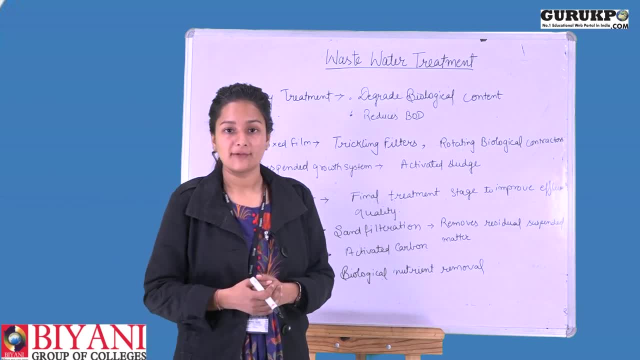 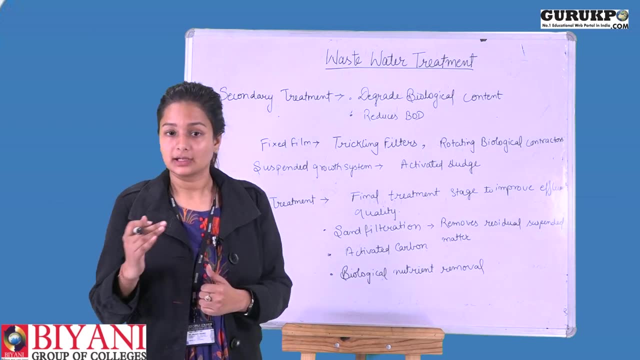 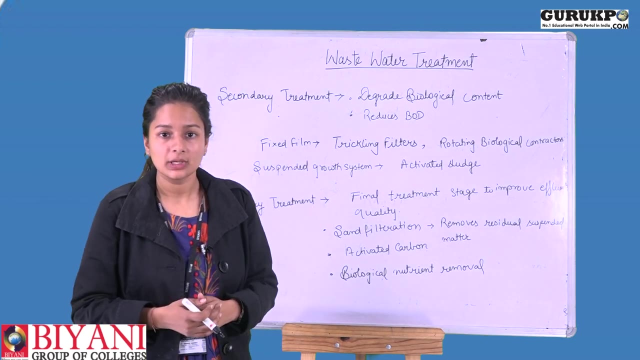 so as we know that polluted water have a high BOD. BOD means biological oxygen, demand means oxygen, the amount of oxygen which is required for the degradation of biological or organic content. so if the organic content would be more, the oxygen demand would be more. so after this treatment, the BOD level 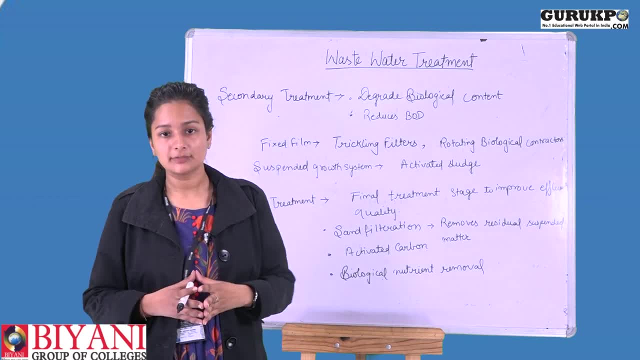 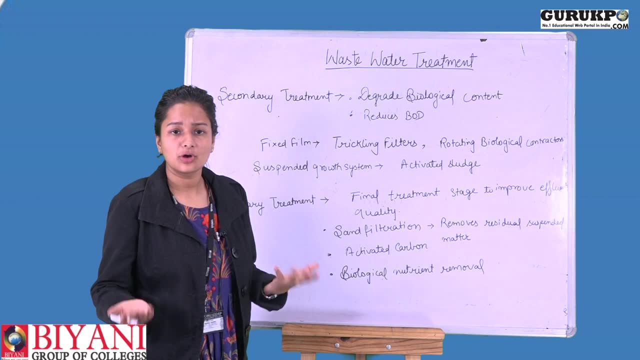 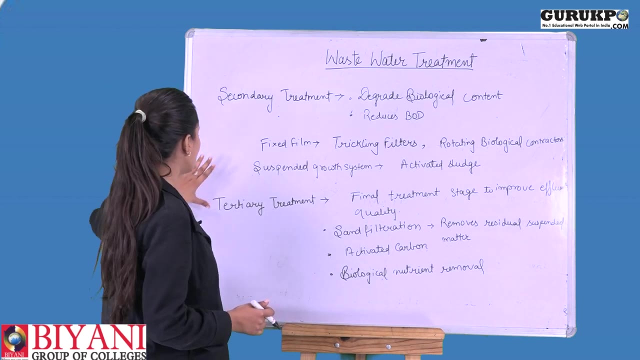 decreases, or we can say 99% of the BOD level we decrease. in this method, we use different types of processes or we can say our tanks. the first comes, and this process is dependent on two things. we can use any kind of biofilm or microbes. 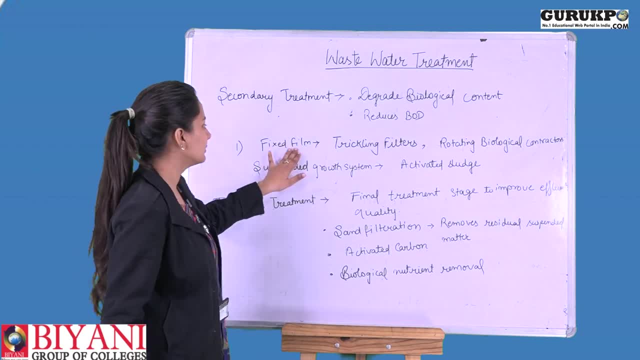 first is fixed water and then we can use any kind of biofilm or microbes. first is fixed water and then we can use any kind of biofilm or microbes. first is fixed film. fixed film means the microbes or the biofilm. biofilm is the sorry biofilm. 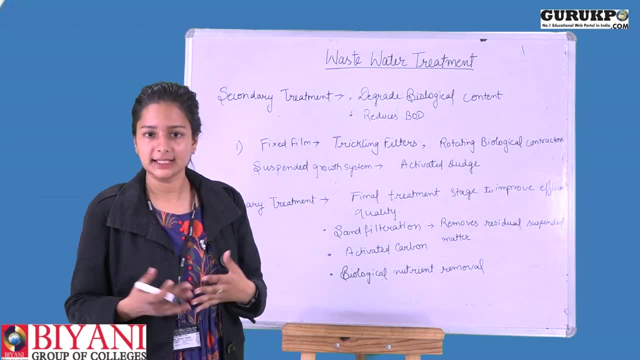 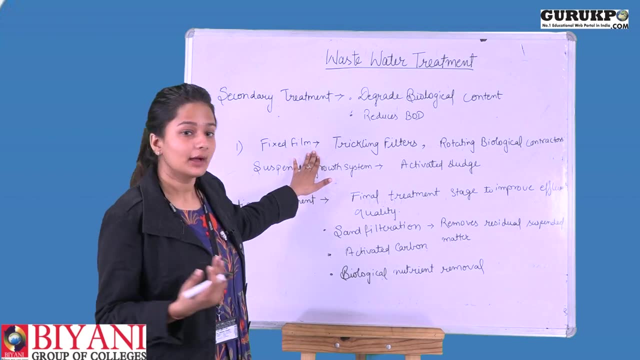 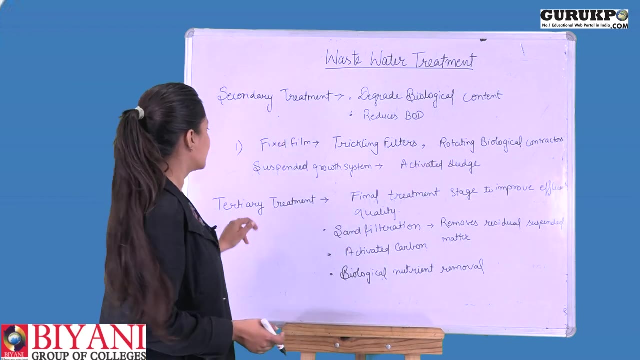 is made up of our microbes, which would further degrade our organic content. so it can be fixed on any rotating disc or any media or any surface, okay, such as trickling filters, rotating biological contractors. next is second is second type is suspended growth system. okay, second type is suspended growth system. 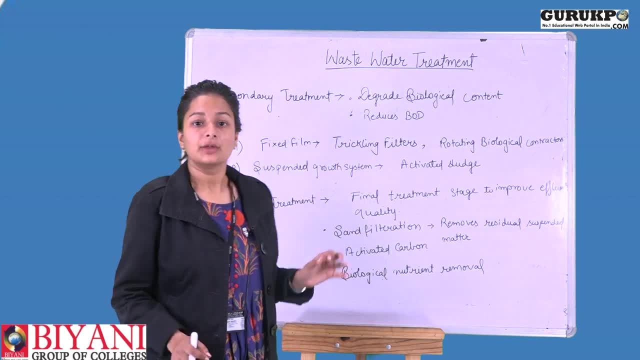 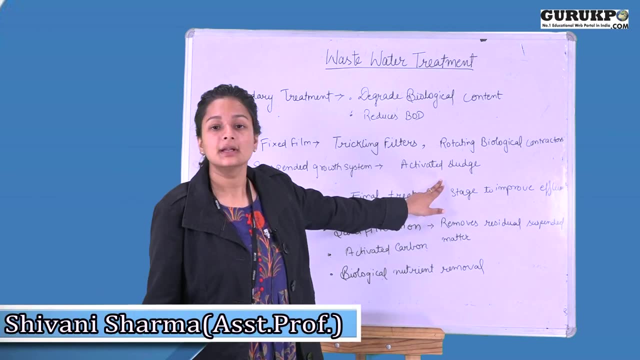 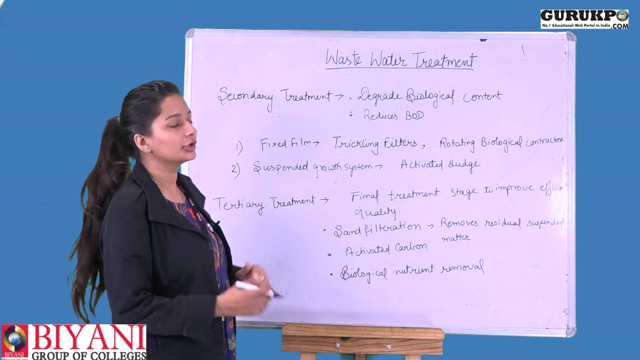 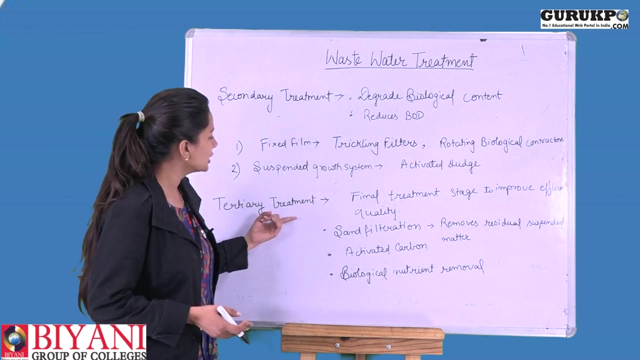 okay, it means we don't use any fixed film. we keeps our biological organisms or microbes in a suspended form, okay, such as activated sludge process. okay, we will further see this method or secondary treatment in detail in the next lecture. so we first jump to the next step, that is, tertiary treatment. it is the final or. 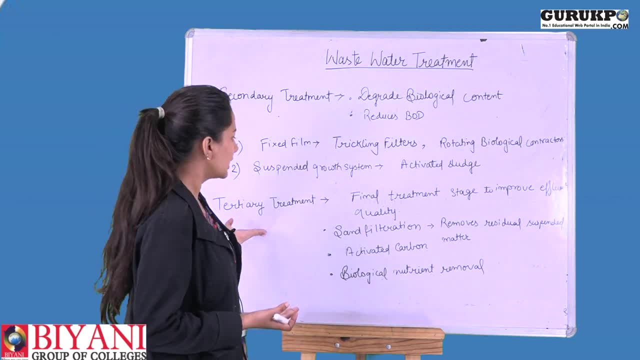 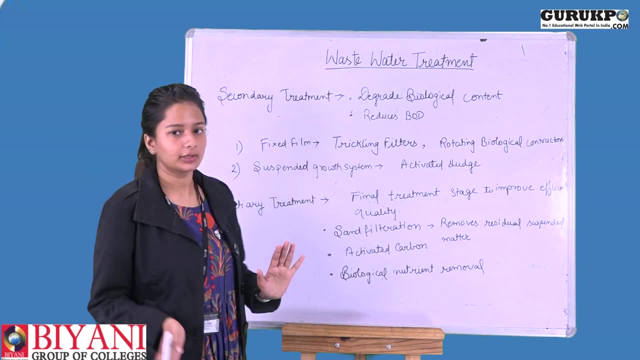 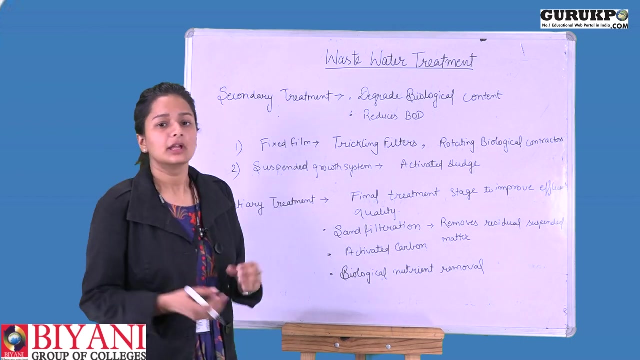 third stage of the treatment process. okay, in this, what we do, we do sand filtration, although we have cleaned our water up to 90%, okay, but still after digestion of by a organic matter we used to get some suspended particles. but secondary treatment k badmai could. 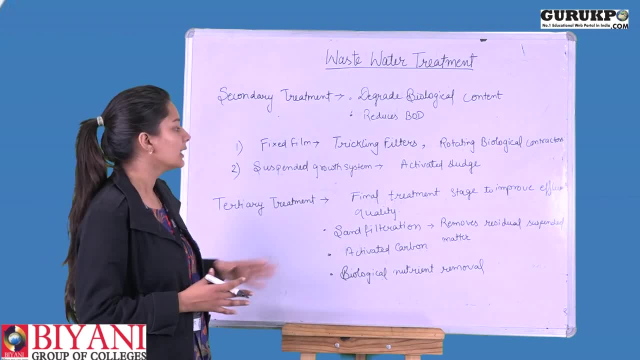 suspended particles. her mariposa cut a house at a heavy continued, so final treatment may have us a water quality going to any-angle. a hum-hum. I got to a hotbructure petal not even don't have got. has lacks. to get it closer still I. these are some that are you can use for at partial is very useful, so on side and achely you can also be able to get and use for other problems that you have been. how to hit the agua. now we see that for in the context of direct exposure to Roja.